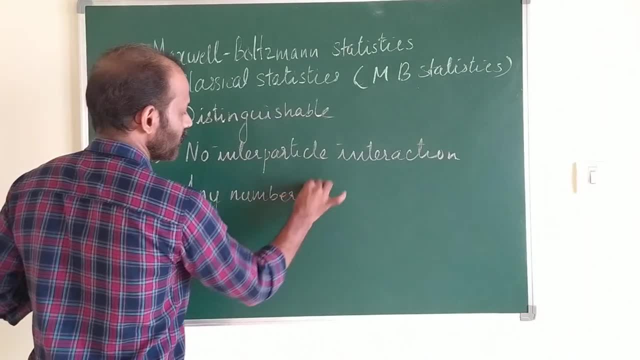 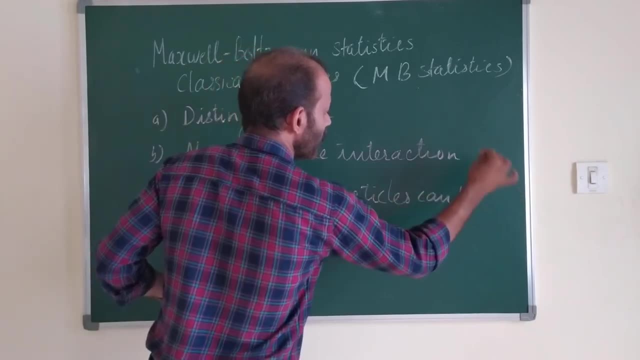 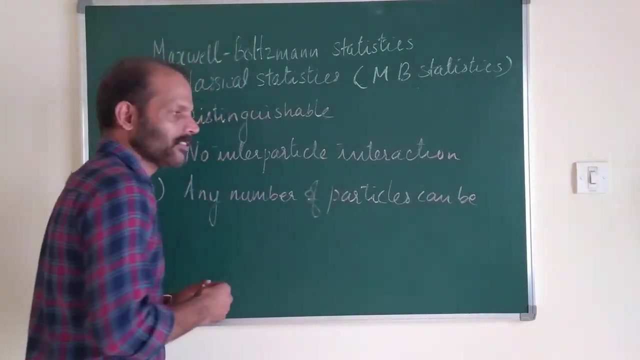 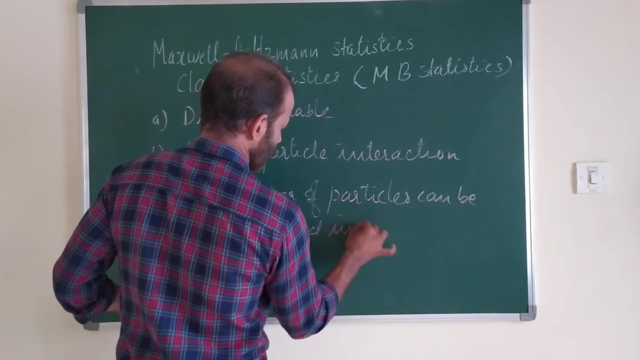 Any number of particles can be accommodated or occupied at a given energy level, Can be occupied in a given energy level. So there are that. The third point is what we are considering here today, Also called energy gradients, perhaps the number of particles. 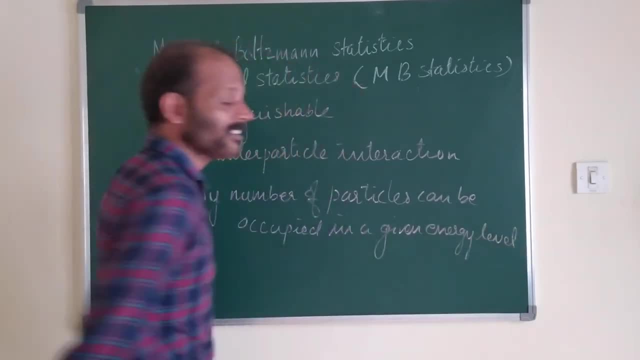 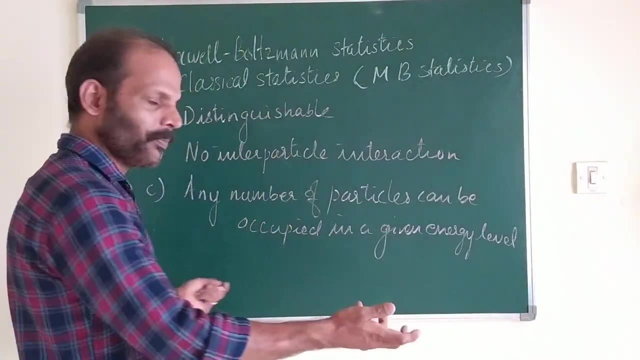 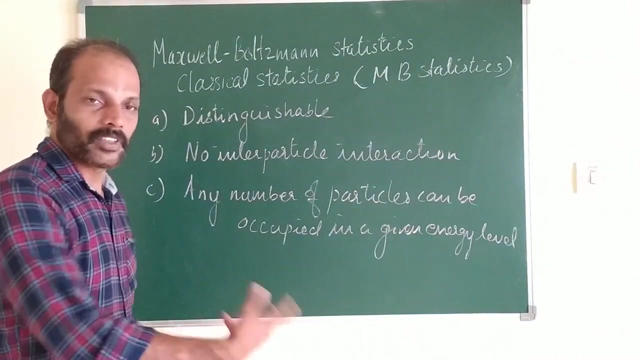 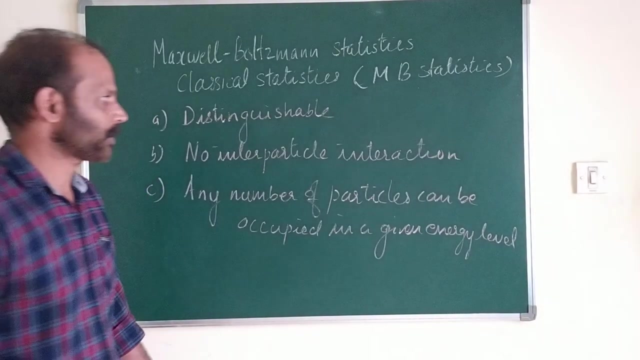 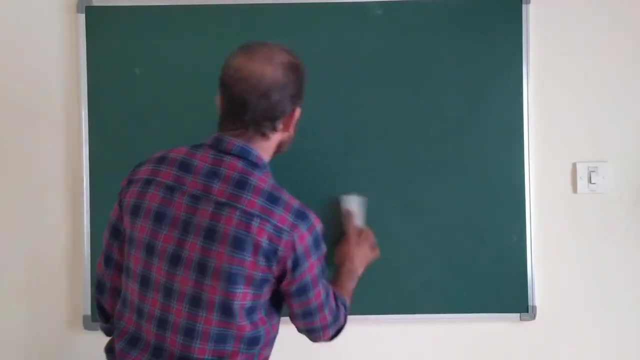 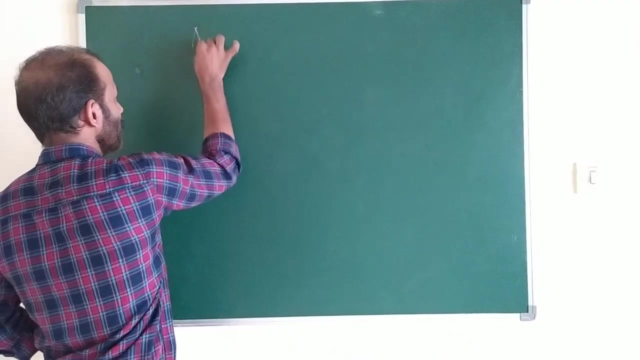 There is no restriction to the particles to occupy or distribute in different energy levels. Any number of particles can be occupied in a given energy level. So we are moving to derive the M-B equation for Maxwell Boltzmann statistics. Consider a system of n particles. 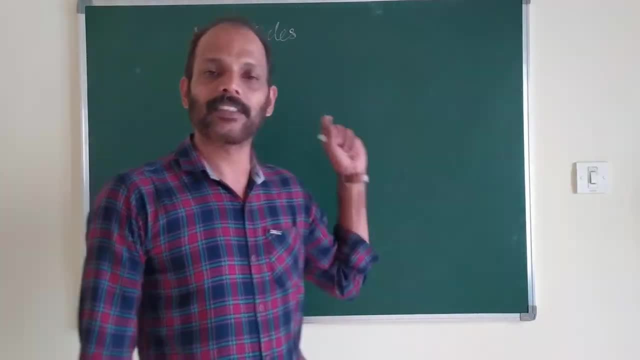 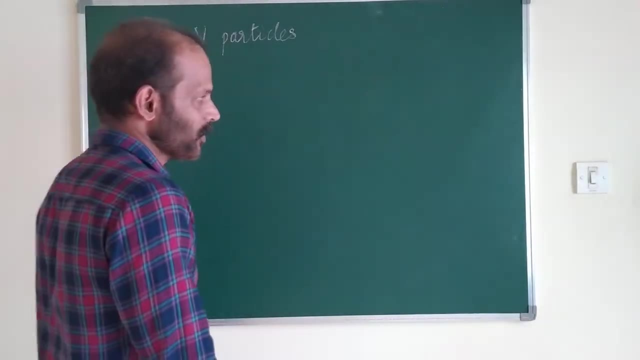 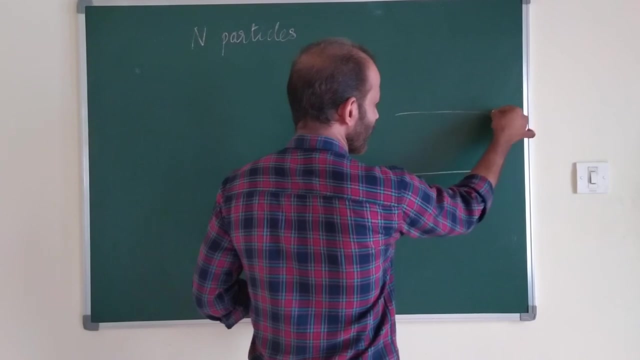 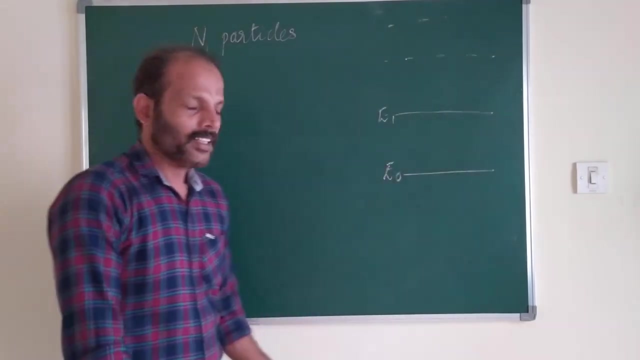 n number of particles. Total number of particles present in the system is n, and among these particles we know, suppose we have one energy level, then second energy level, suppose it is E0, it is E1, so and so and so, then E0 can accommodate few particles. 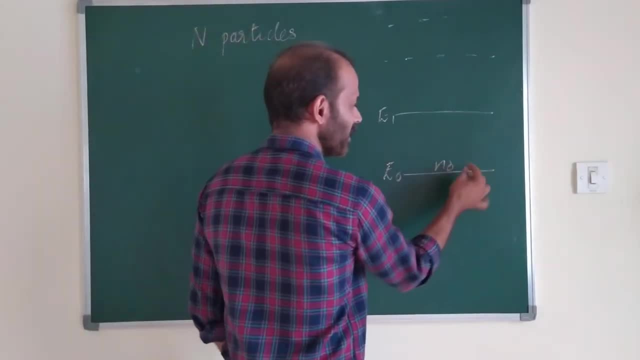 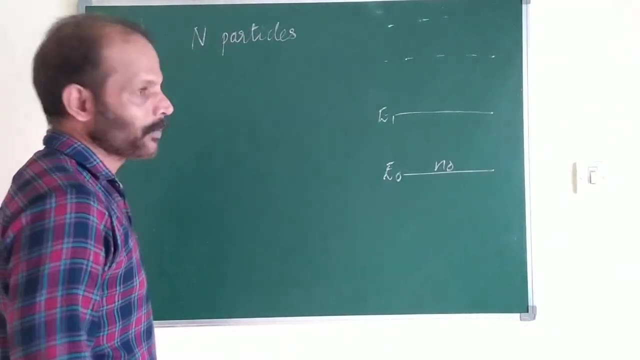 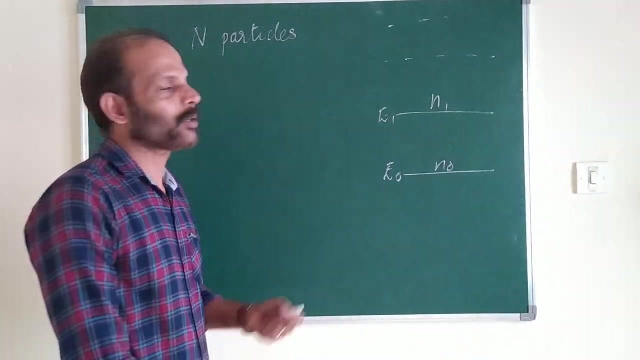 Suppose it is n0, that is n0 particles are occupied. then second level is E0, ground level. E0 is occupied by n0 particles, then it is n1 particle, then E2 level is occupied by n2 particles. so and so, so the particles are distributed. 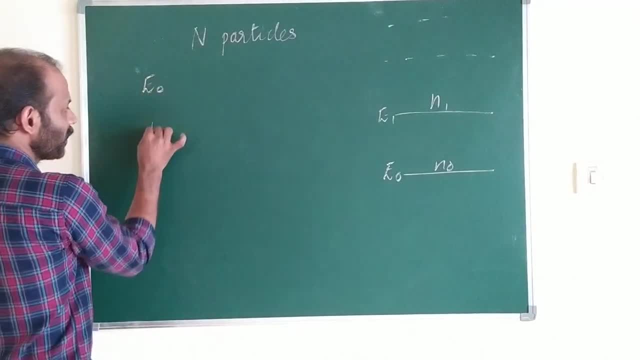 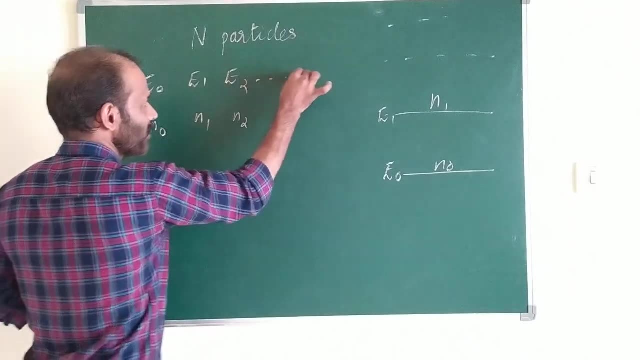 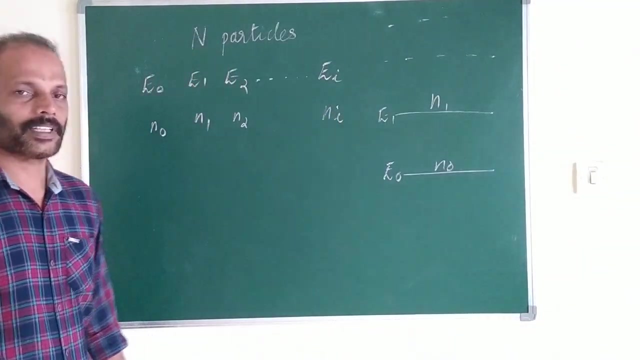 in such a way that E0 level contains n0 particles, E1 level contains n1 particles. E2 level contains n2 particles. so and so. so the number of particles present in E1 level is nn. for the sake of simplicity, we are not considering the D-Helm scheme. 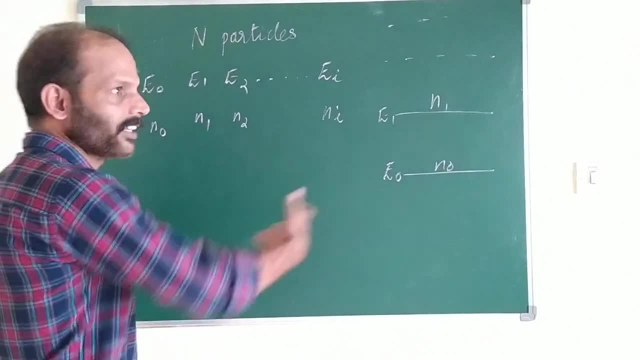 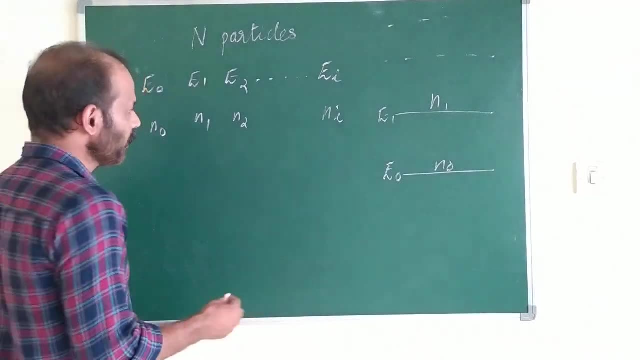 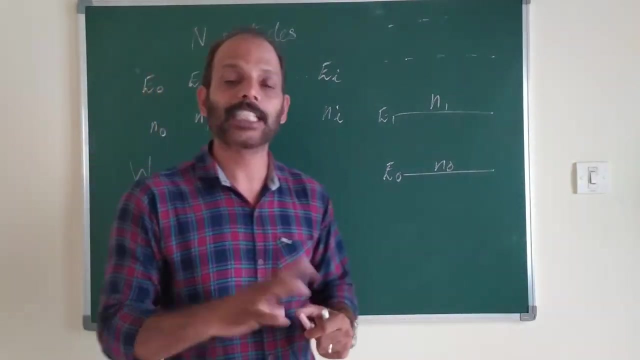 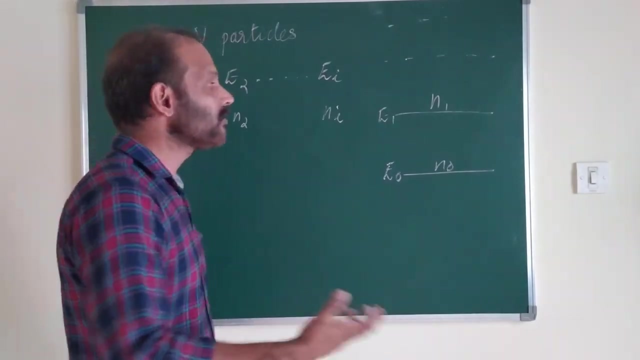 in the very beginning. we can include it later. so the thermodynamic probability W, we already discussed it. that is, it is the maximum. E0, that is, it is the maximum way of distribution of particles in a system. it is the maximum number of ways the particles are distributed. 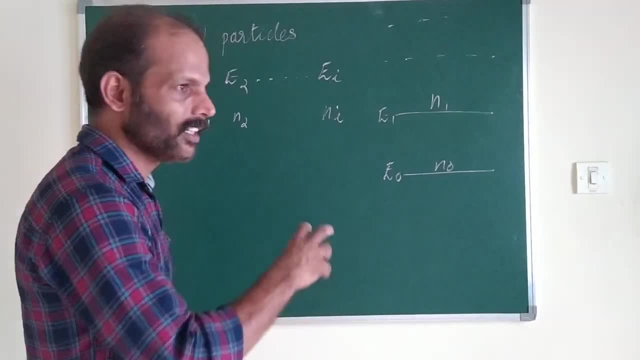 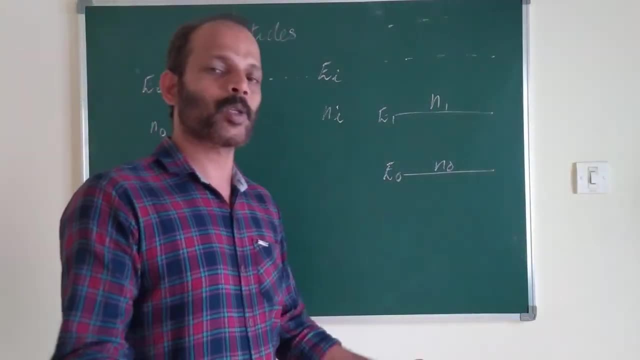 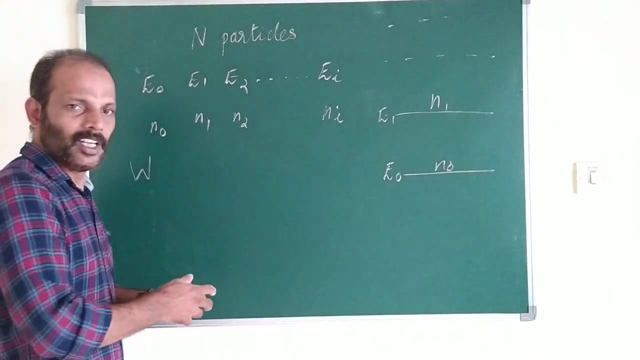 in different energy levels. that is thermodynamic probability, and we know the maximum ways of distribution of particles. it is also known as the micro states of the system. so simply, this W means thermodynamic probability. so by determining W we are actually determining micro state of a particular macro state. 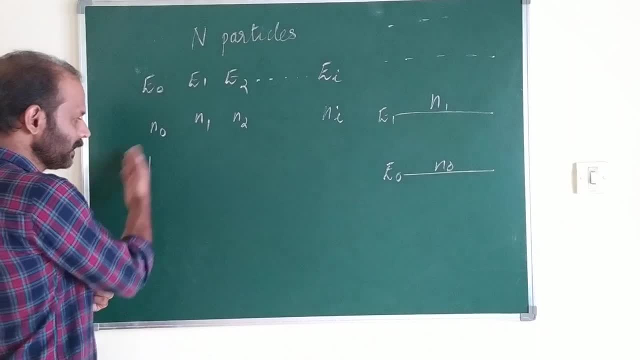 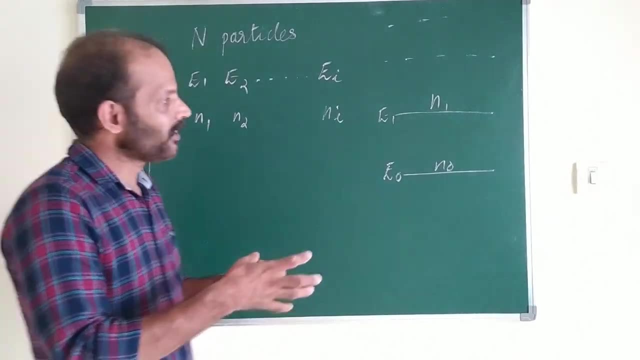 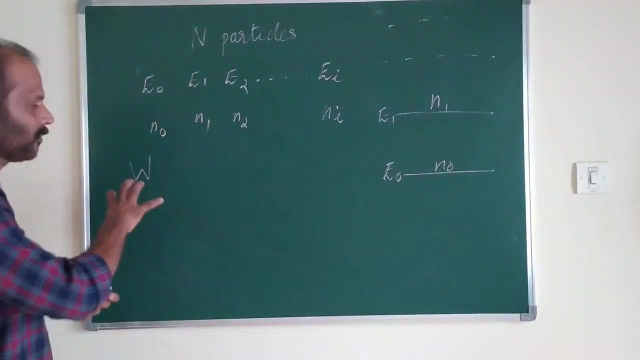 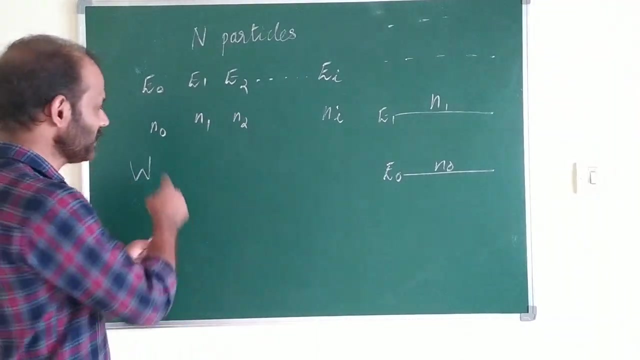 right, because it is the maximum probability. maximum ways of distribution. how many ways nn number of particles can be distributed in different energy levels of a system? that is W, the maximum value, the maximum way by which the nn particles are distributed. it is W and the same thing. 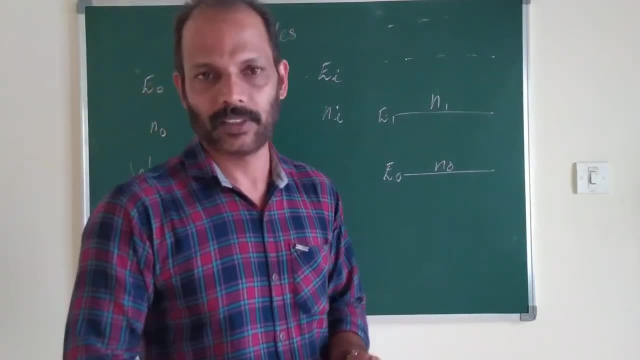 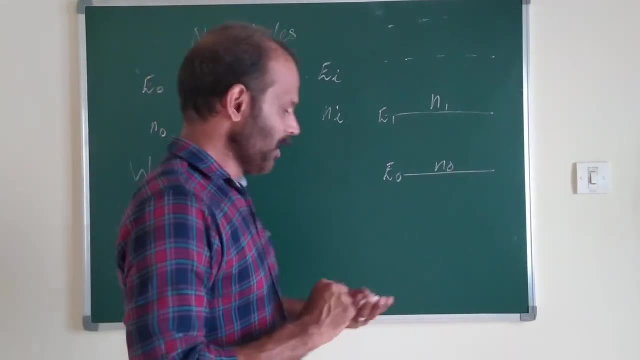 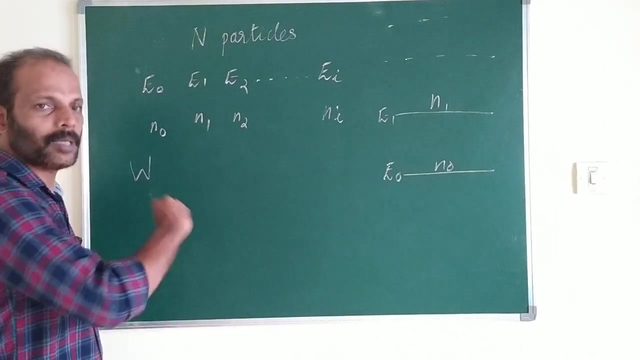 is micro state because it is again different types of distribution. so by calculating W we are actually calculating micro state, micro state of a given macro state. so what is our aim is to calculate W, calculate thermodynamic probability, that is, maximum thermodynamic probability, or the number of 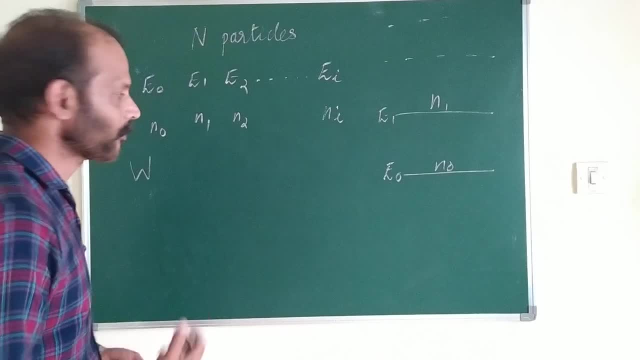 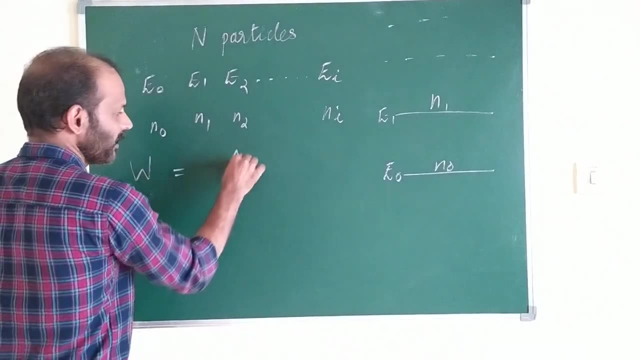 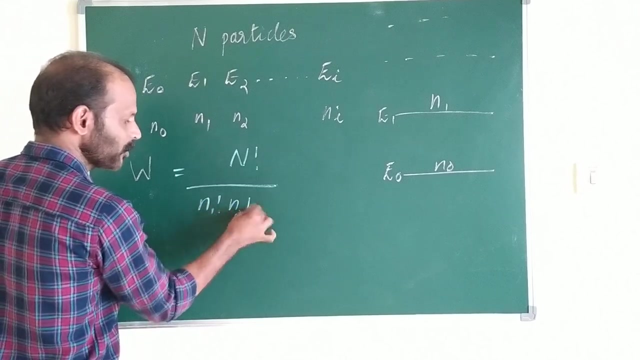 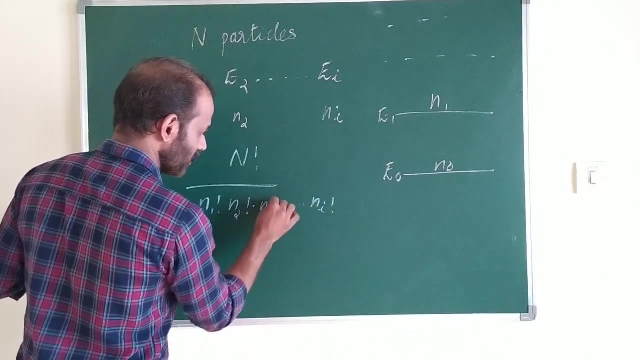 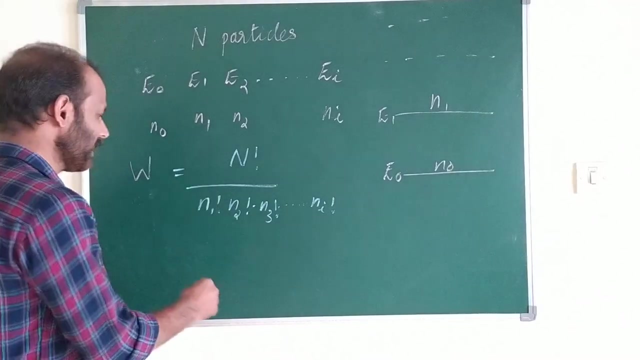 micro states for a given macro state. that is the way. so here these are. so W can be given as n factorial divided by n1 factorial times n2 factorial times n3 factorial, and so ni factorial, ni factorial, ni factorial. it is actually a product. so we can write it as: 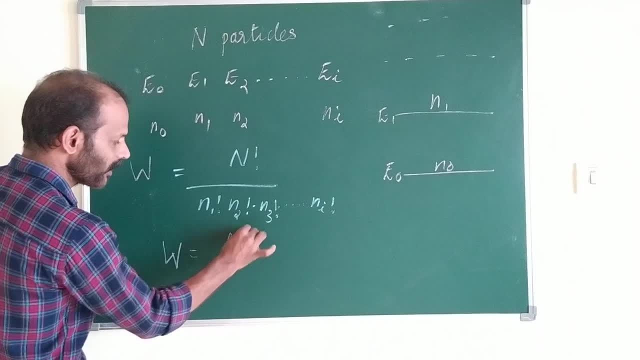 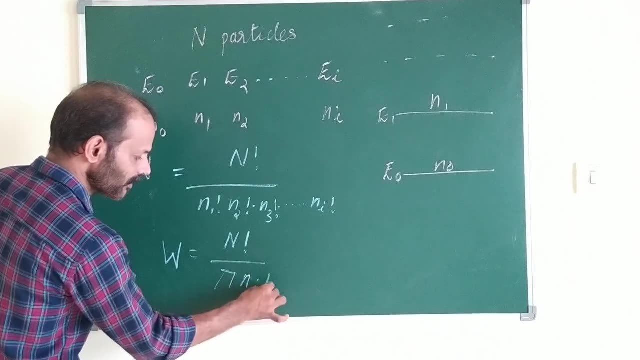 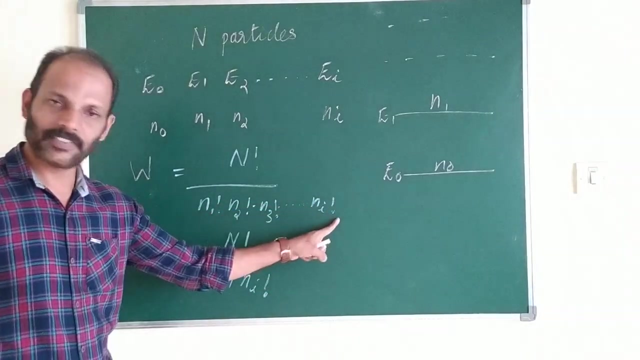 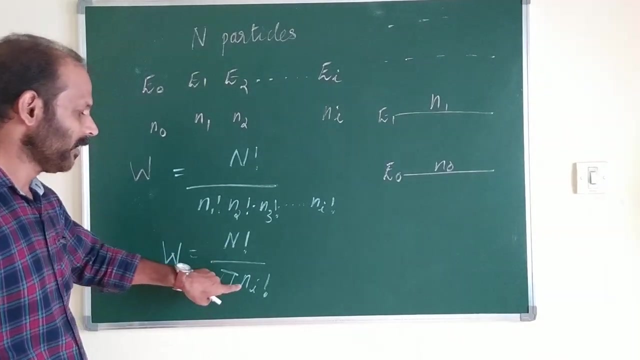 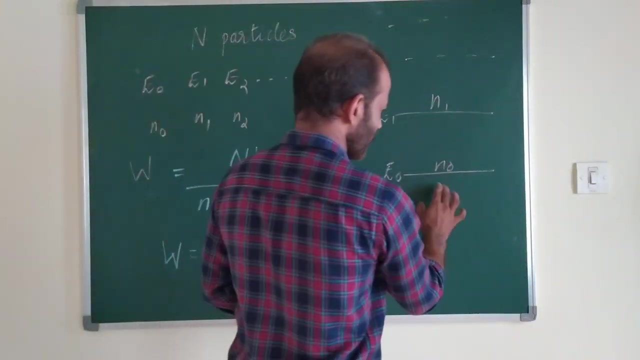 W is equal to n factorial divided by capital, pi ni factorial. pi is the product of these numbers, these factorials, pi. so W can be written as W is equal to n factorial divided by pi ni factorial. now we can consider the these levels. suppose these levels contain sub levels. 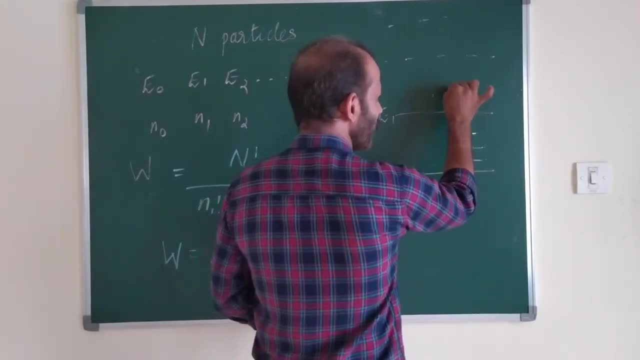 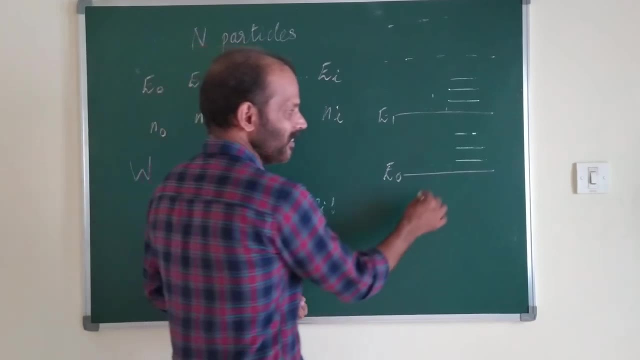 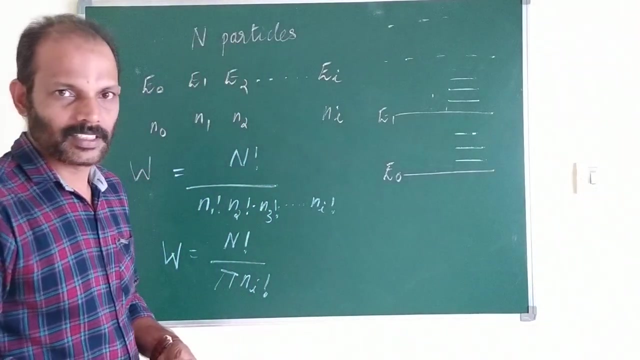 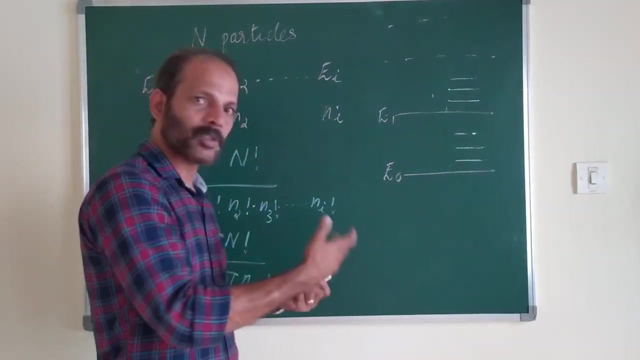 suppose this contains three sub levels, or this contains four sub levels, or maybe three sub levels. whatever it may be, then n0 particles can be accommodated on all these sub levels. also, when sub levels are available, particles or atoms or molecules may be occupied in the given. 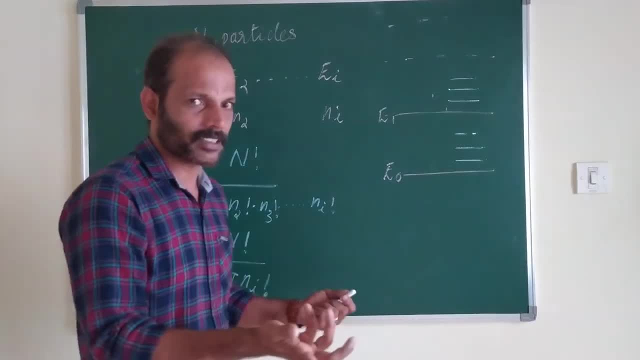 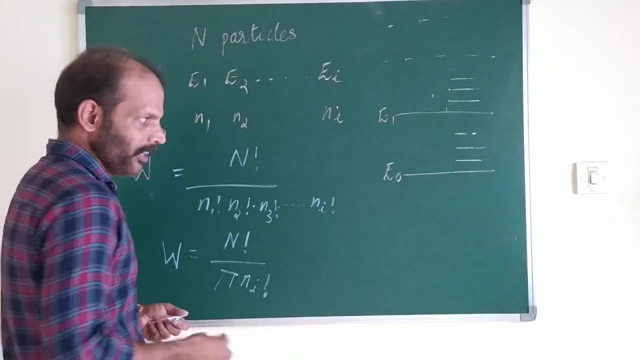 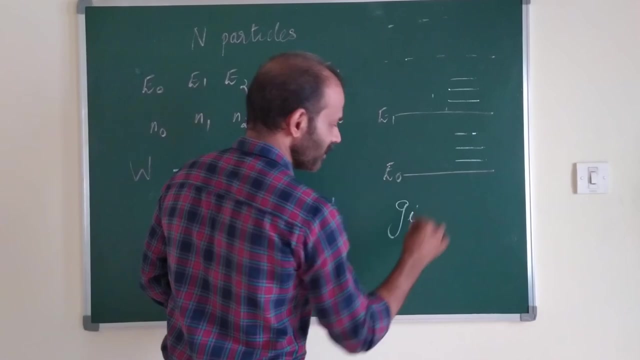 or in the available sub levels. also we call it as multiplicity. so multiplicity is the distribution of particles in different sub levels available. if e0 contains this much sub levels, suppose the number of sub levels is gi, we can call it as degeneracy. we can call it the number of sub levels are degeneracy. 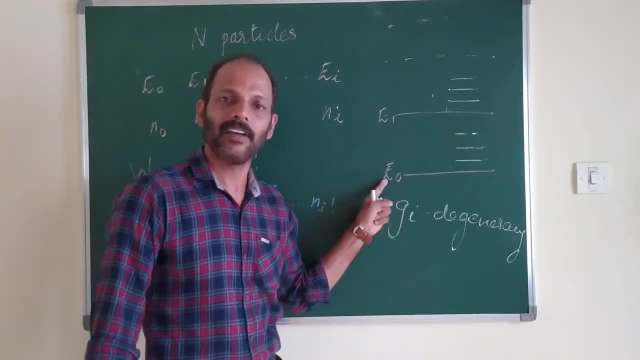 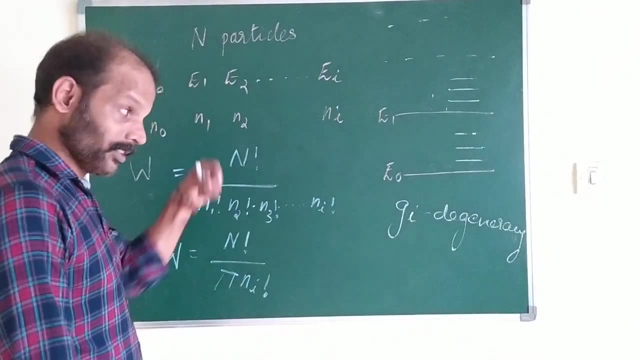 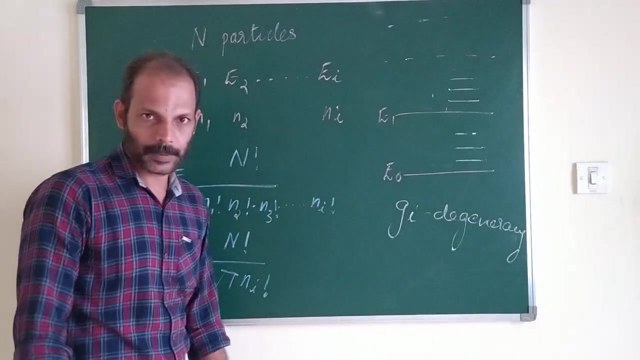 number of sub levels means all these sub levels are the same energy. so it is known as degeneracy of the degeneracy of the energy level. so particles can also be accommodated in all these sub levels. so if gi is the degeneracy and it has only one, 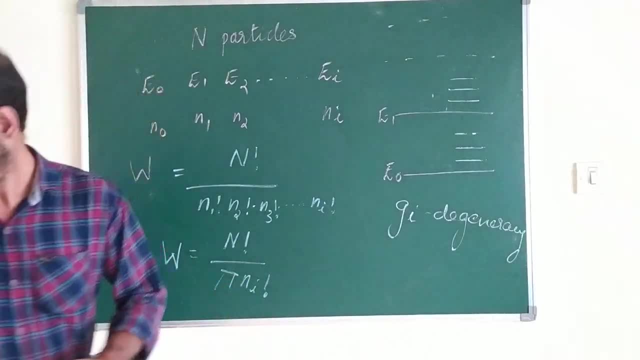 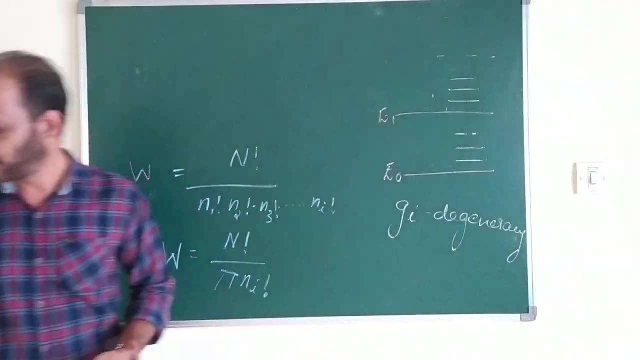 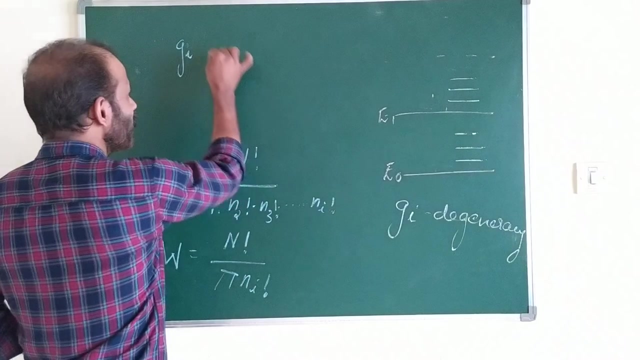 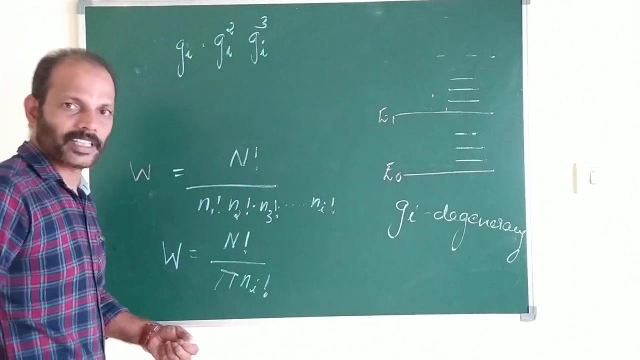 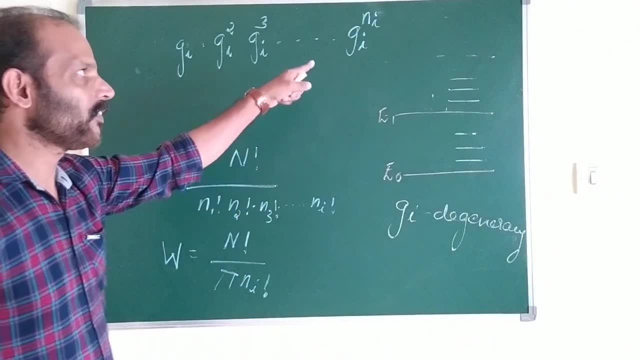 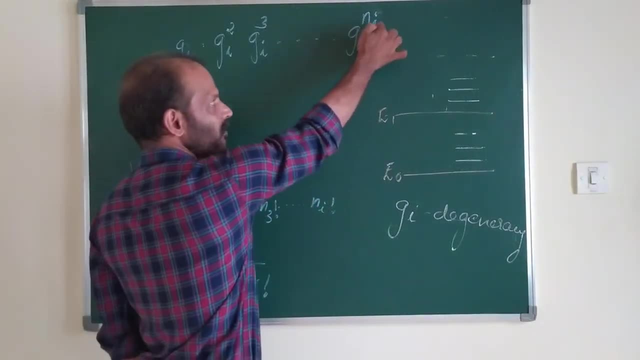 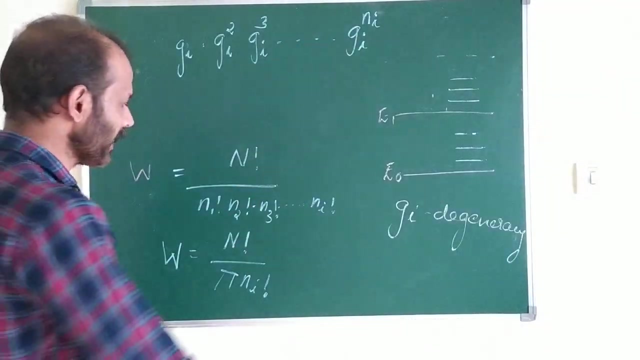 it is gi rise to number of particles ni. that is the maximum possible ways of arrangement of different particles, that is number of ni particles in gi levels for arrangement of ni particles in gi sub levels, gi degeneracy. so it is again a product, so we can include the degeneracy also. 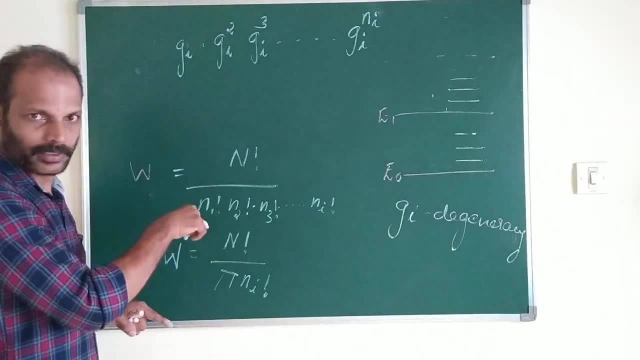 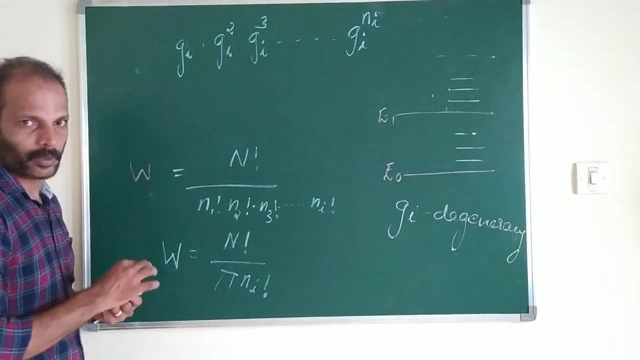 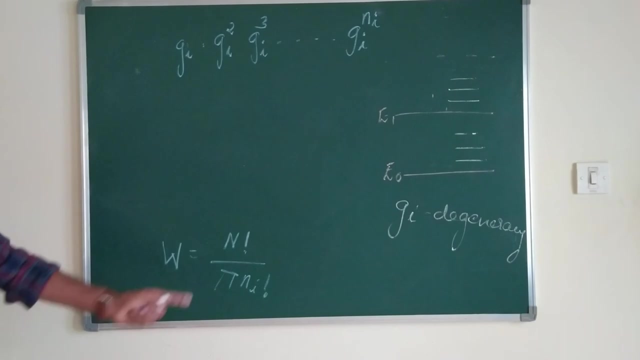 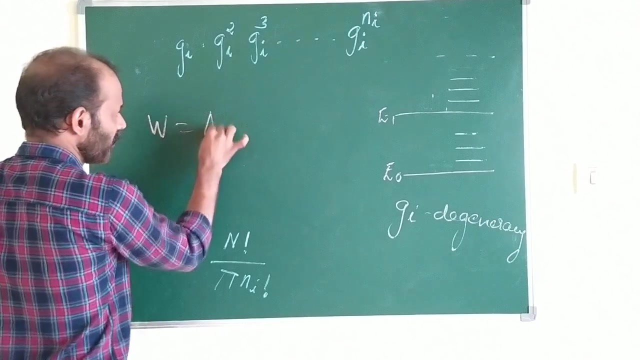 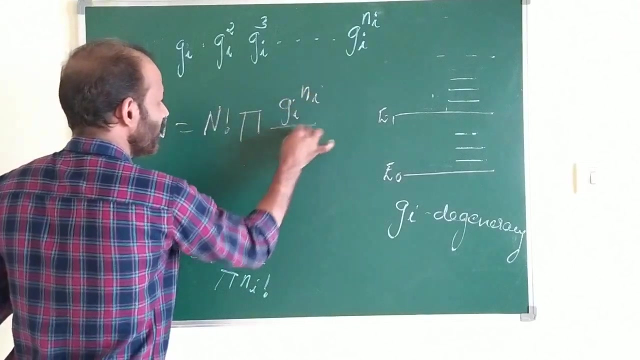 in our thermodynamic probability equation. we can also include gi rise to ni in our w equation, so we can rewrite this equation as we can rewrite this equation as w is equal to n factorial pi. gi rise to ni divided by ni factorial pi is common to both numerator and the. 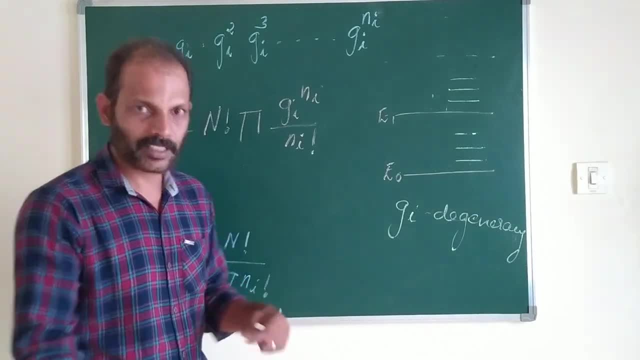 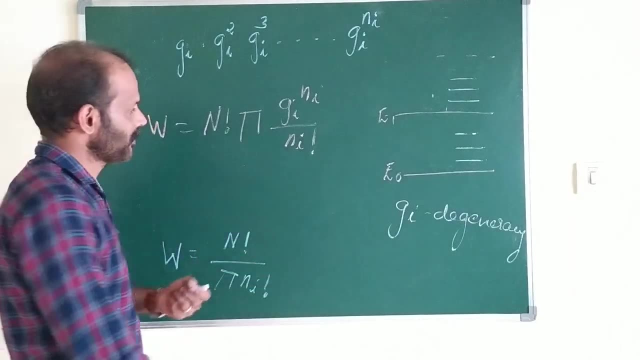 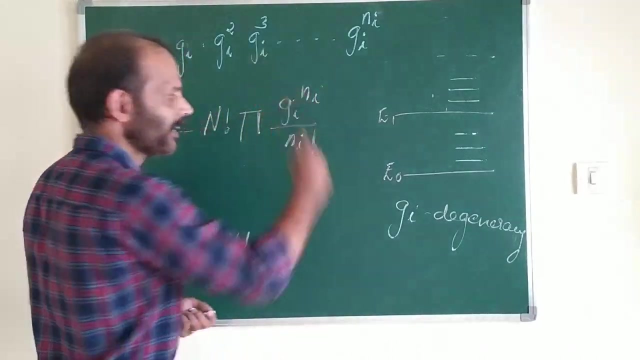 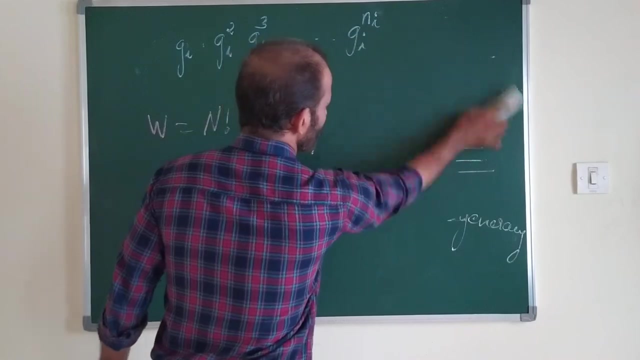 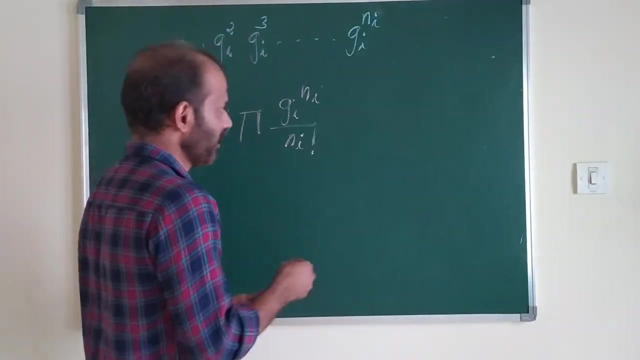 denominator, because both are products and n is constant, so there is no product function or summation, so it is constant. so it is pi gi rise to ni divided by ni factorial. and one more thing is that there is a relation between entropy and thermodynamic probability, that is, entropy s is equal. 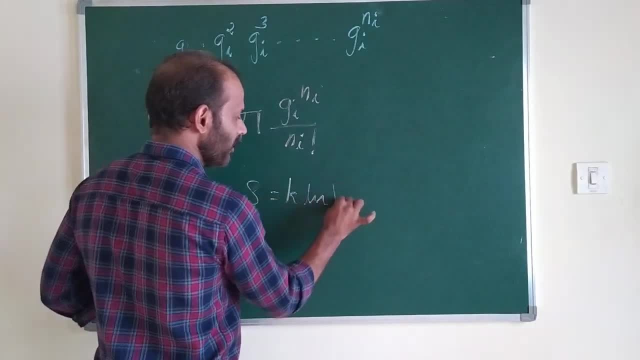 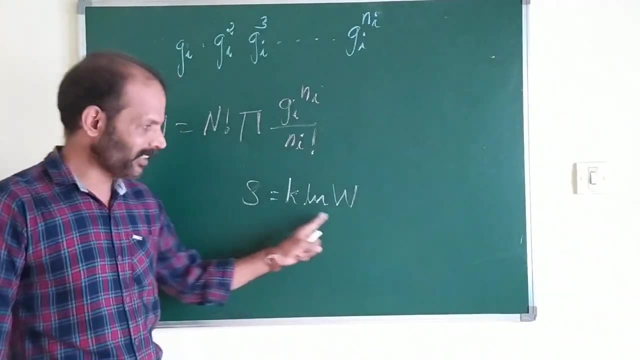 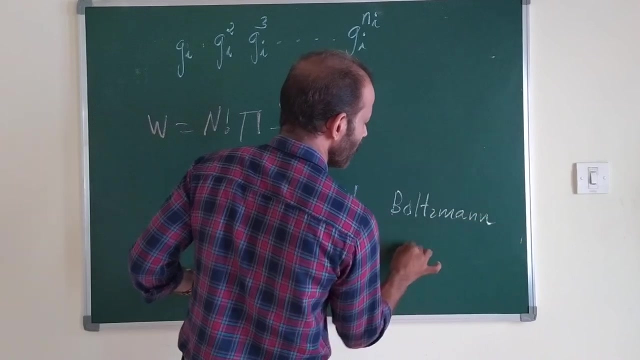 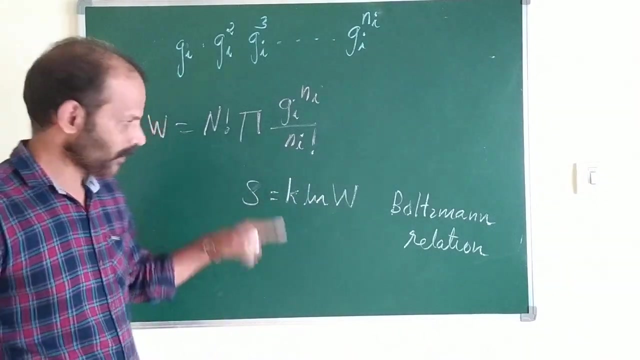 to k, ln, w. this is the relation between entropy and thermodynamic probability and it is known as Boltzmann relation, Boltzmann relation or Boltzmann equation. we will derive this equation later in this chapter itself. it is the relation between entropy and thermodynamic probability. 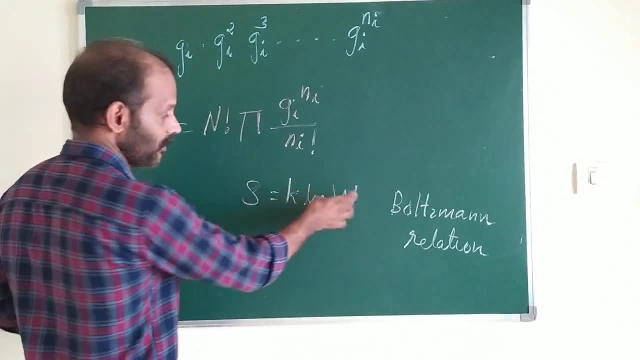 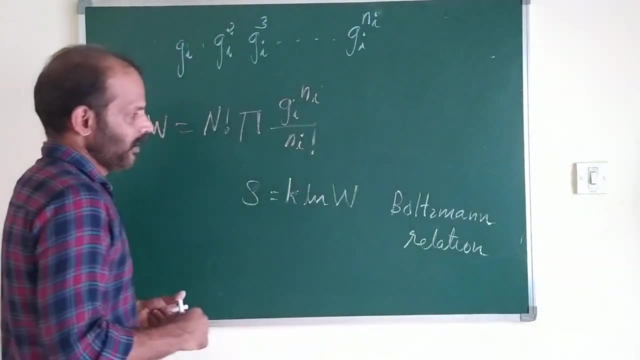 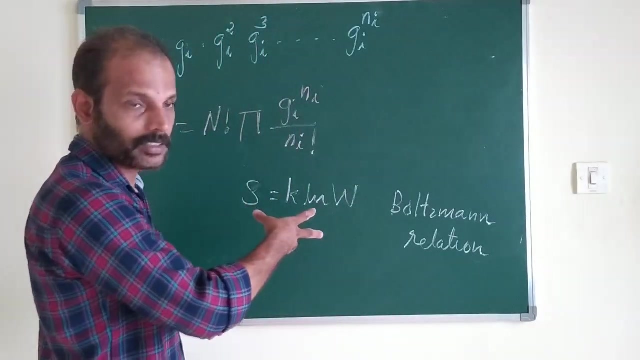 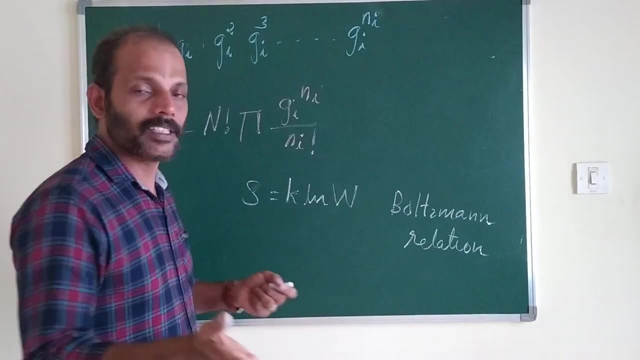 so we are having maximum probability by calculating w we can. that is, the maximum probability is possible at the equilibrium. actually, why maximum probability is at equilibrium, maximum probability, maximum thermodynamic probability, I mean maxim thermodynamic probability- is at equilibrium because thermodynamic probability is the distribution of particles. 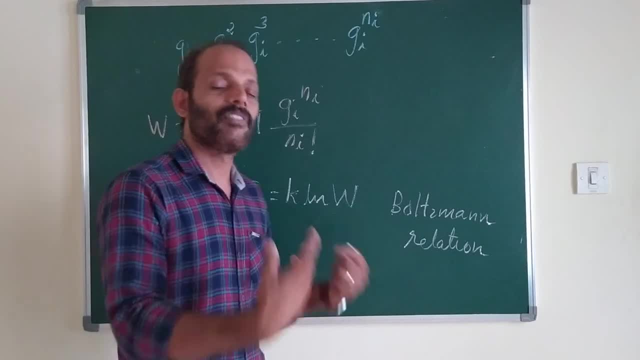 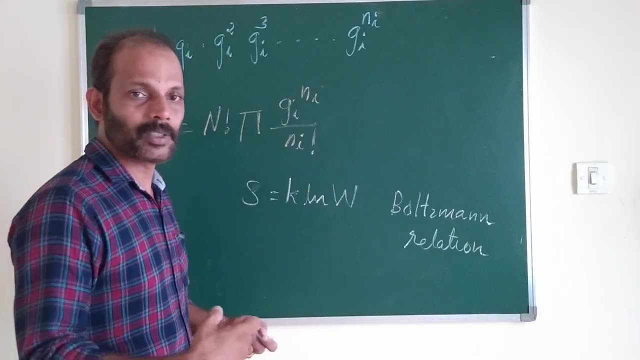 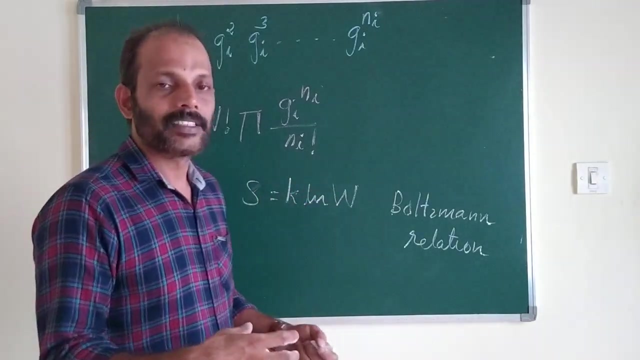 in different energy levels. maximum ways, how many ways the particles can be accommodated, can be distributed respectively in different energy levels. that is maximum at equilibrium, because when a system attains equilibriel And if the system attains equilibrium, then there is no more different arrangements possible. 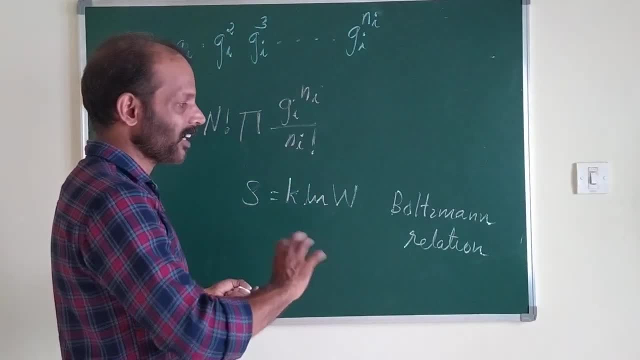 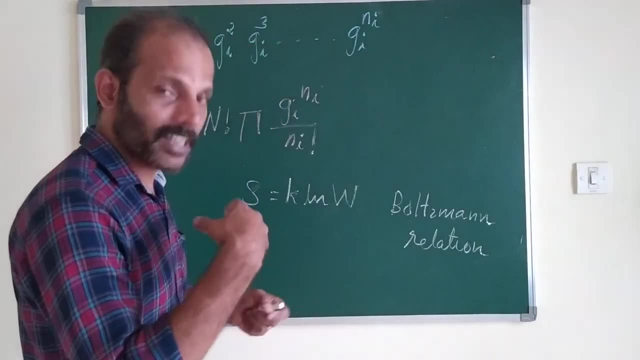 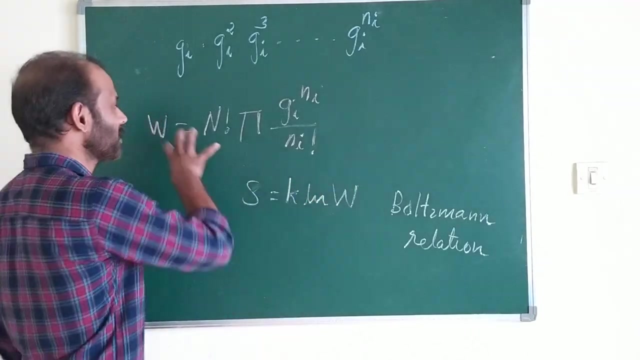 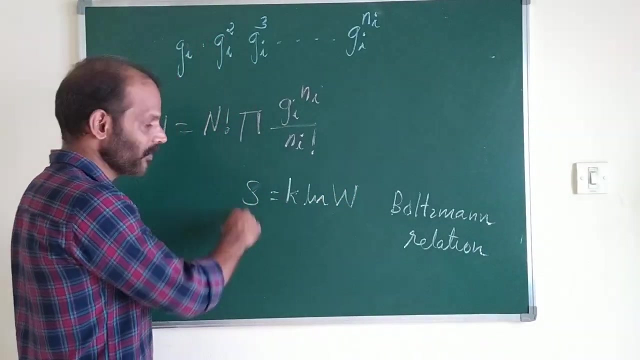 Maximum changes having already been done. So there is no more different changes after attaining equilibrium. So the maximum possible ways of arrangement, that is, maximum thermal dynamic probability, is at the equilibrium. Okay, so just keep in mind that this relation should be between entropy and the thermal dynamic probability. 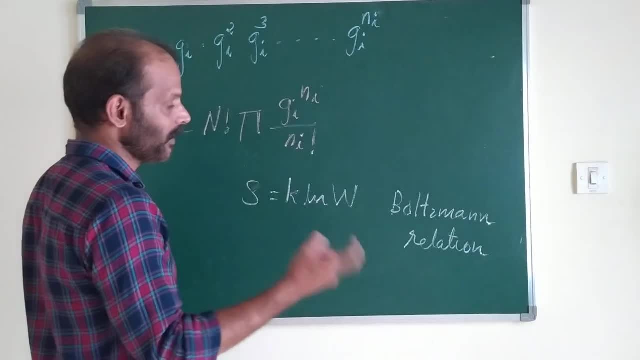 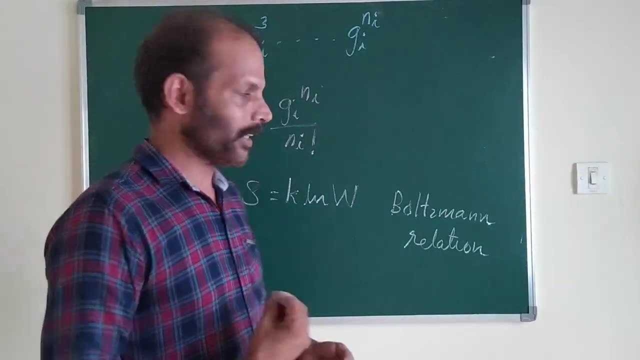 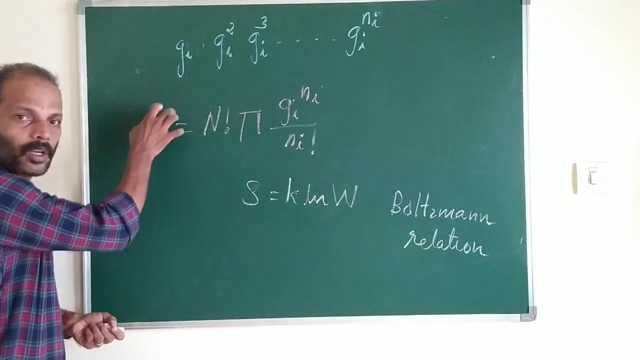 And thermal dynamic probability, maximum values of thermal dynamic probability. it is at equilibrium. When a system attains equilibrium, it gets maximum value for thermal dynamic probability. Then, in order to calculate W, just, we are taking natural log of this W. 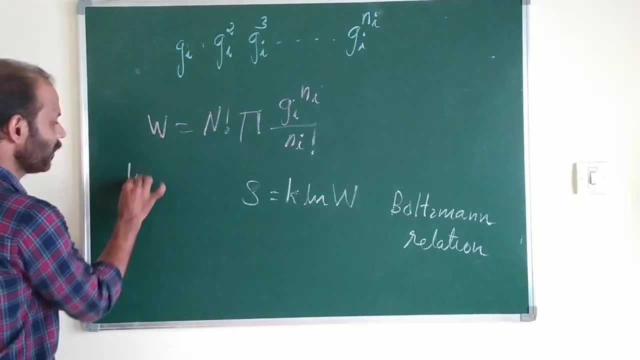 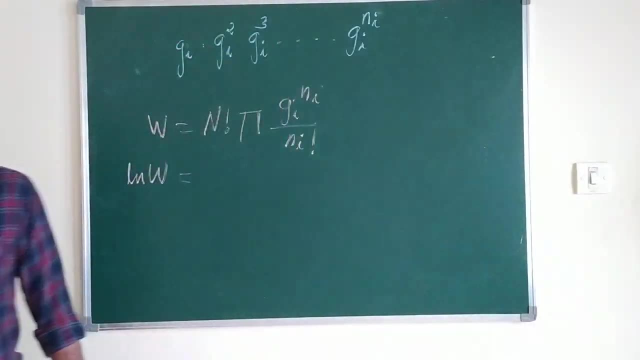 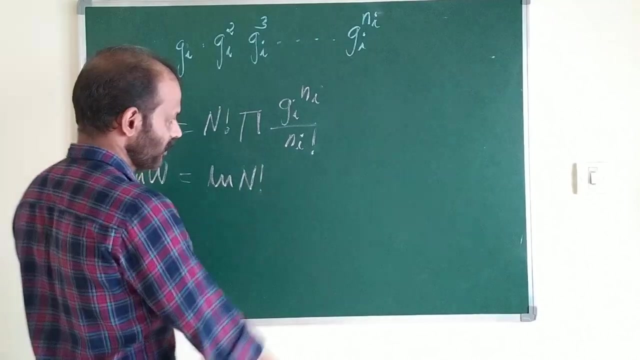 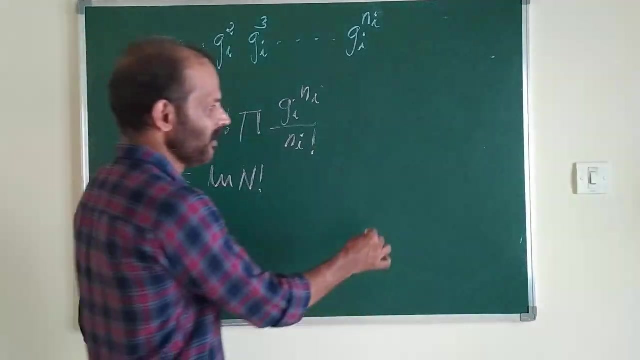 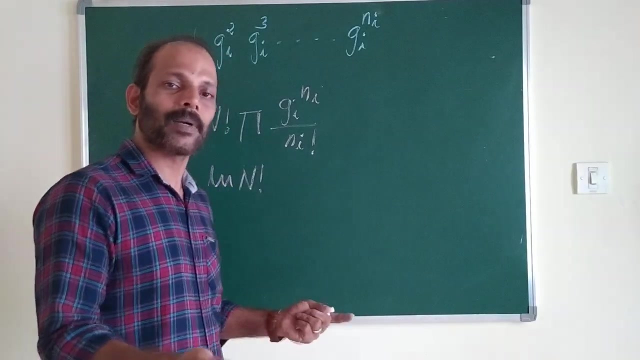 That is ln W W equal to ln n factorial. Then when we are taking log n, the product becomes summation, For example log A times B or log A into B, which is equal to log A plus log B. So the product. 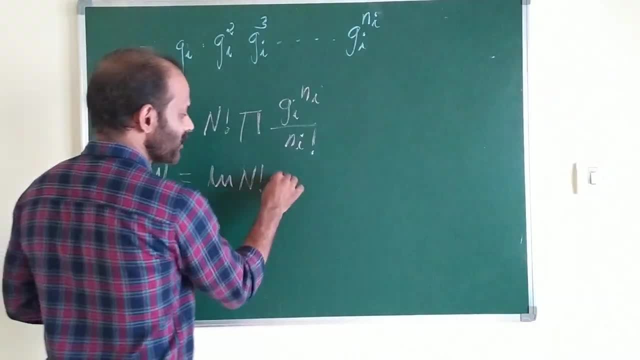 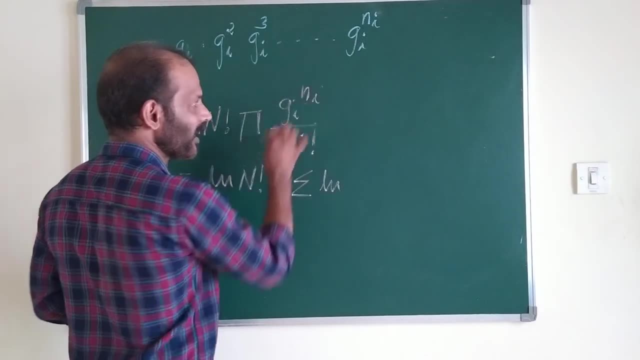 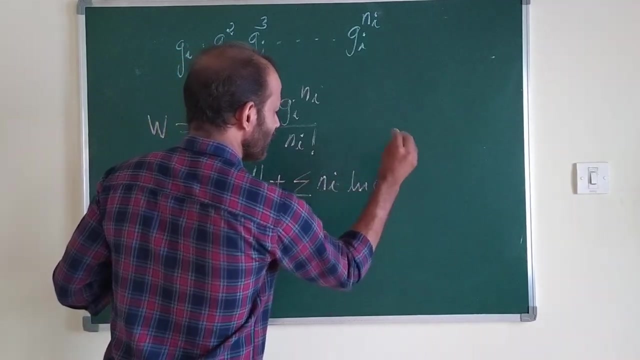 So we are replacing this by summation, that is, sigma ln g i rise to n i. We can write it as n i ln g i. ln g i rise to n i is equal to n i g i. n i ln g i. 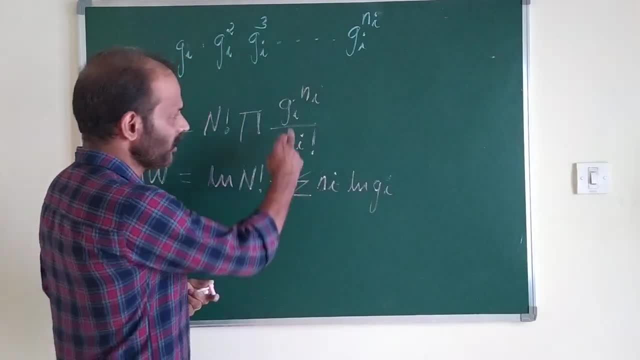 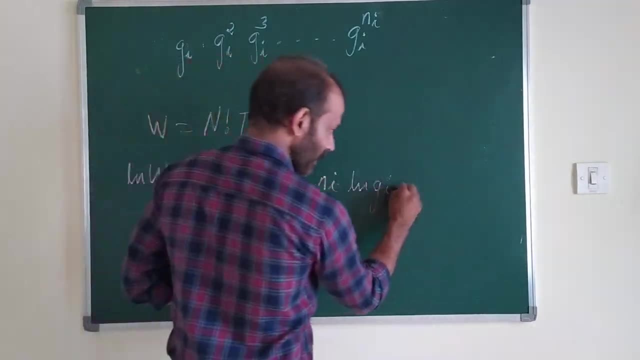 Log x rise to n is equal to n log x. It is the same formula, So ln g i n i is equal to n i n i l n g i. Then it is numerator, so it becomes minus. That is log A by B. 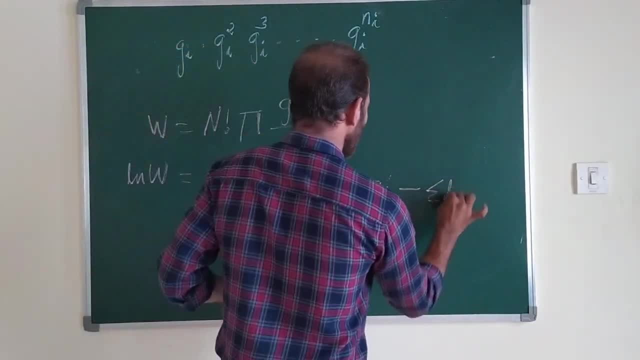 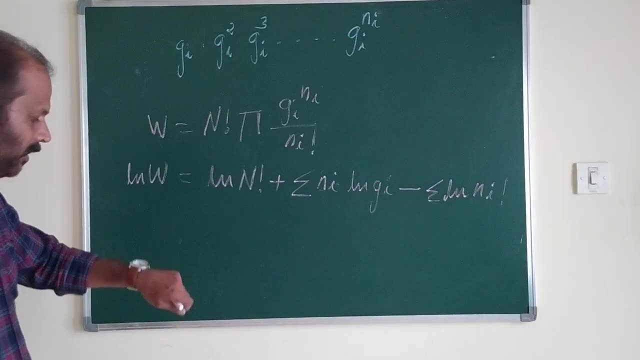 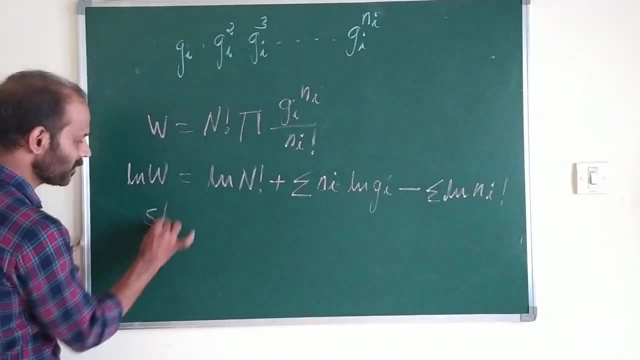 That is log A minus log B. So sigma ln, n i factorial. That is our equation. This is our equation for thermal dynamic probability when it is taken in log A. And we are expanding this equation By using Stirling's approximation. 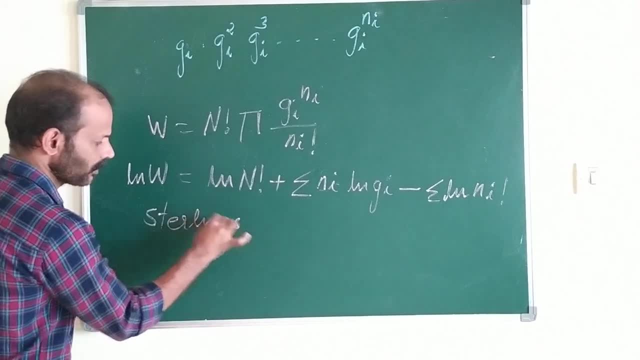 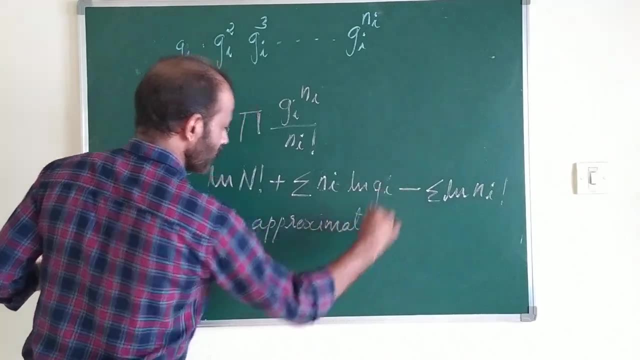 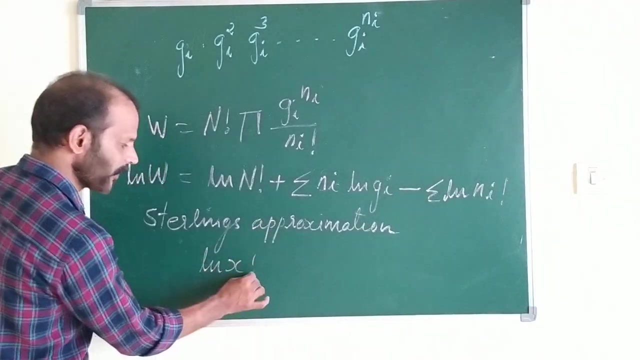 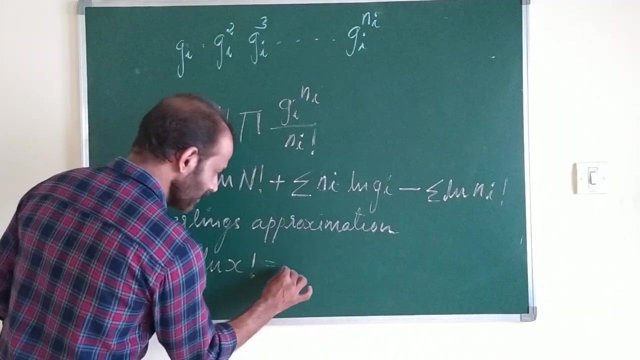 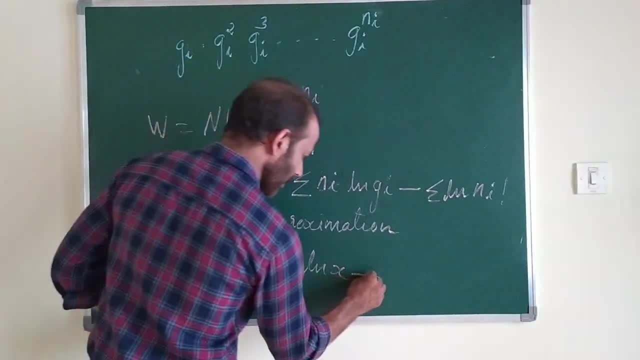 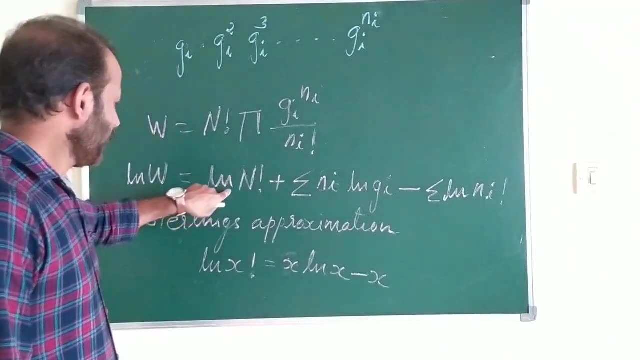 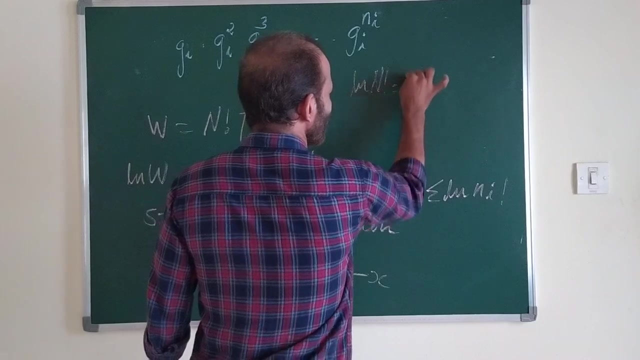 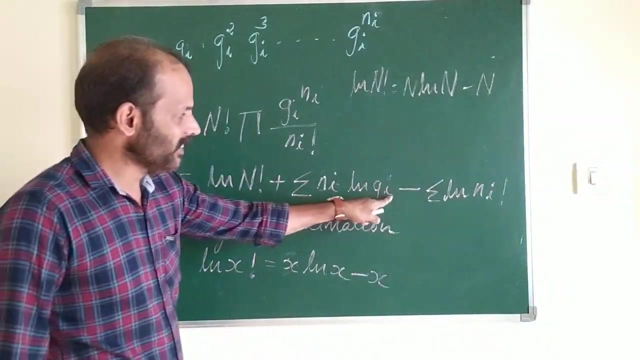 x, ln x, x, ln 2.. We can apply this right x x, ln x minus x, x, ln x minus x. that is our sterling's approximation. So ln n factorial is equal to ln n. factorial is equal to n. ln n minus n, Then ln gi, which is equal to gi. 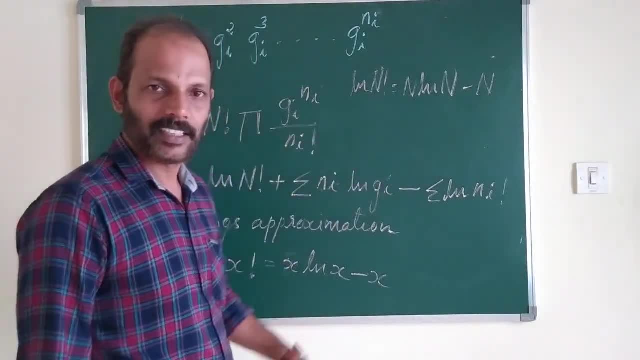 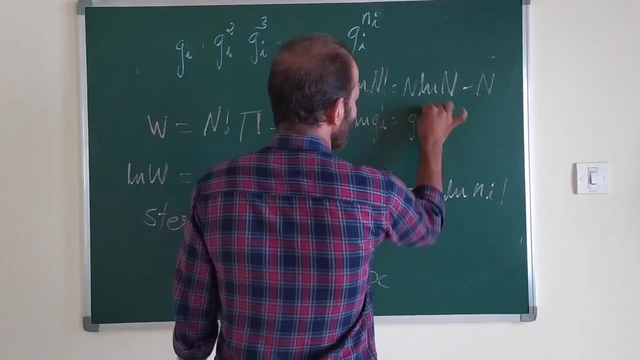 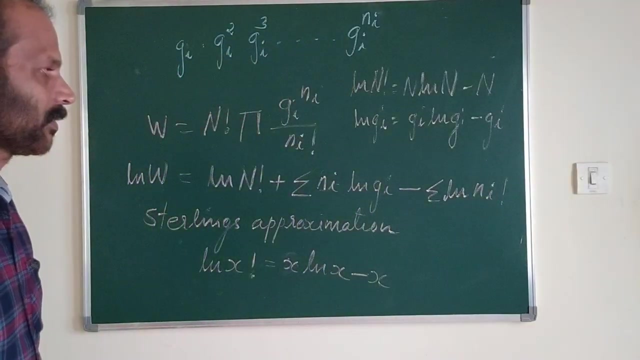 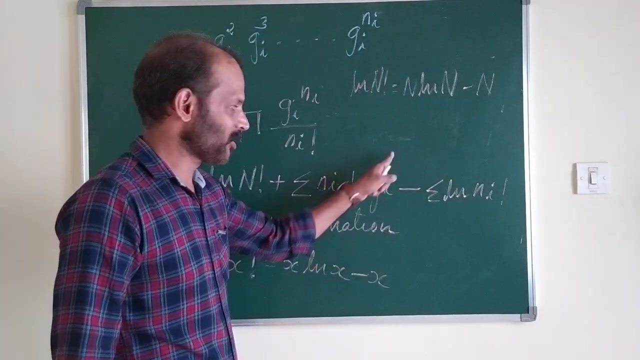 ln gi minus gi. that is, ln gi is equal to gi. ln gi minus gi. Right, Sorry, We do not need this gi because there is no fact. okay, Sorry, So we do not need that step. So the next one. 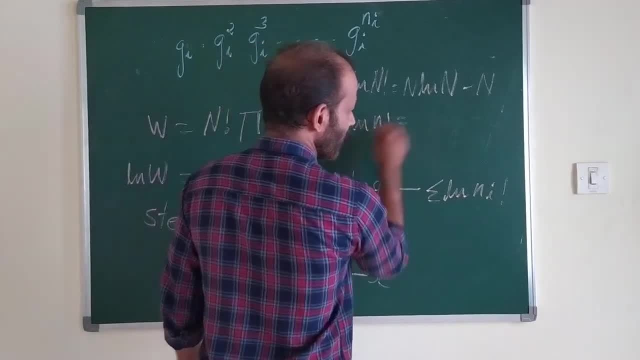 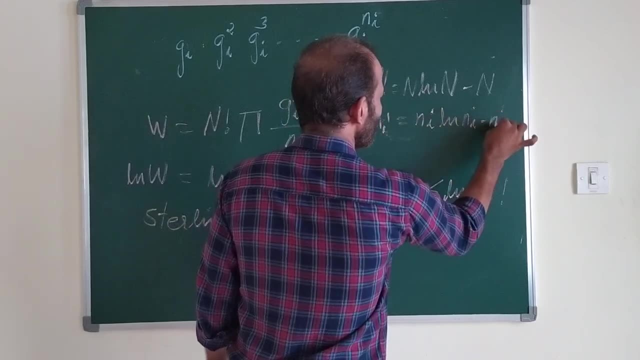 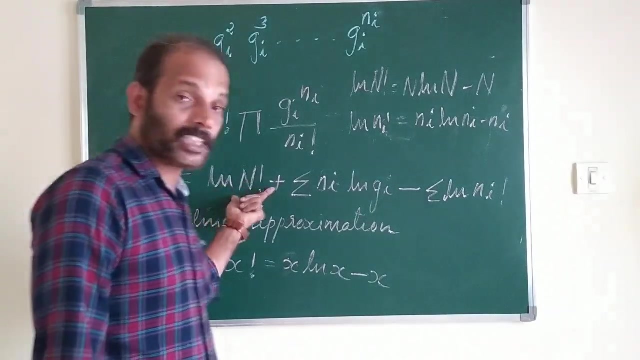 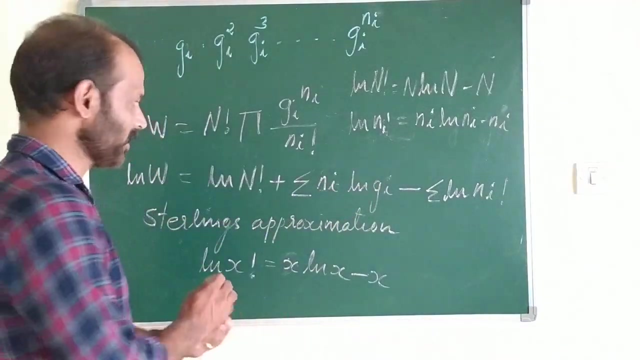 That is ln n factorial, which is equal to n i, ln n i minus n i. So we need only two expansions, that is, ln n factorial and ln n i factorial. These two expansions can be done using sterling's approximation, So substituting values of ln n factorial and ln n i factorial. 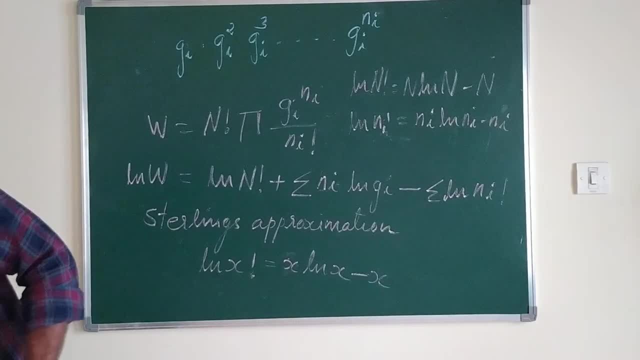 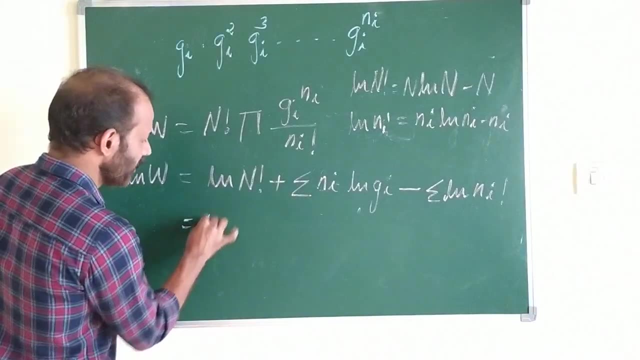 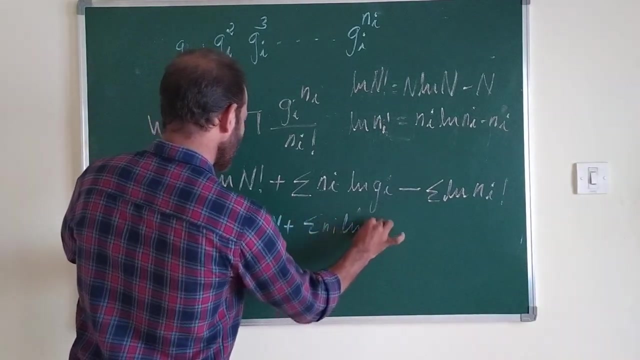 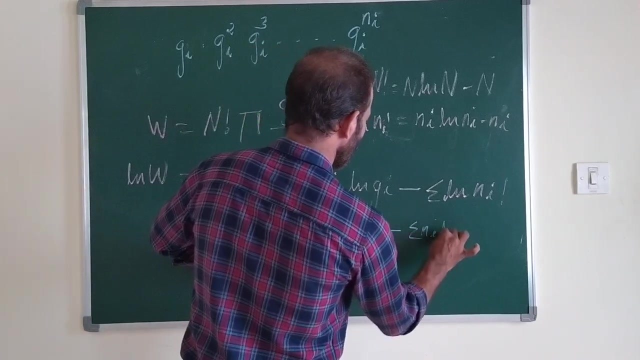 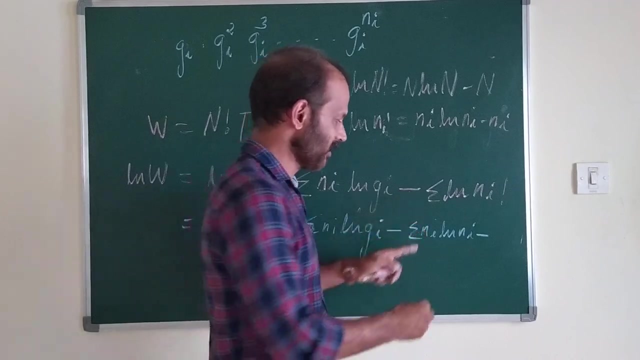 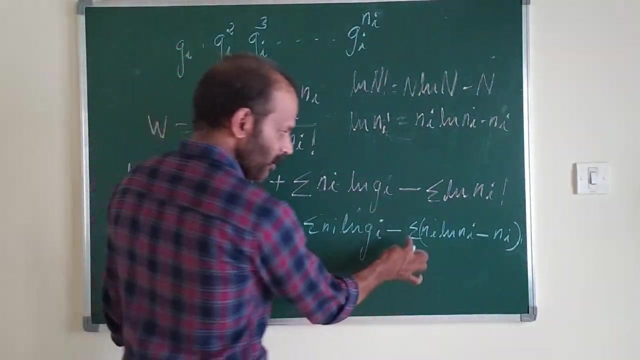 in here, Okay, And in here we get…. … which is equal to n ln n minus n, plus sigma n i ln gi minus sigma n i ln n i minus. Then again 2 minus Okay, Okay, that is minus n I okay. so this minus Sigma into minus n I become plus Sigma. 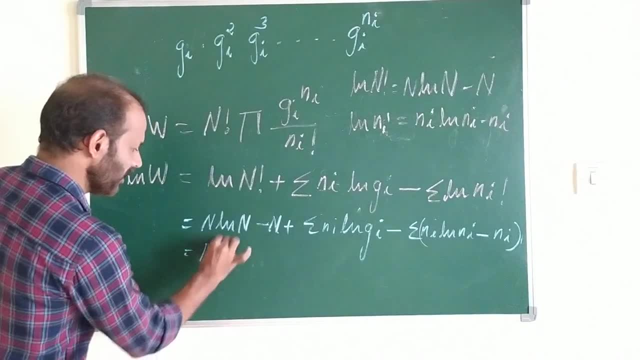 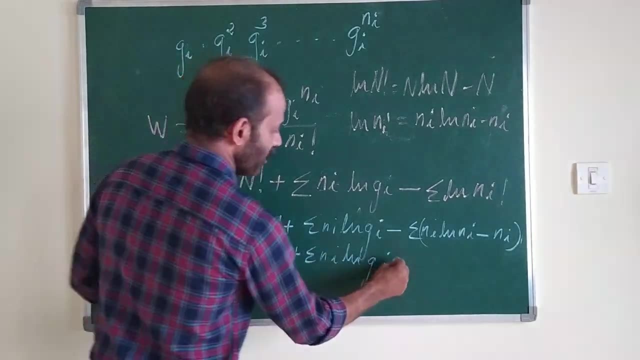 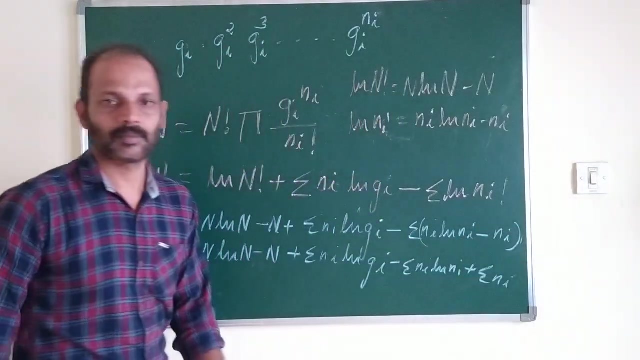 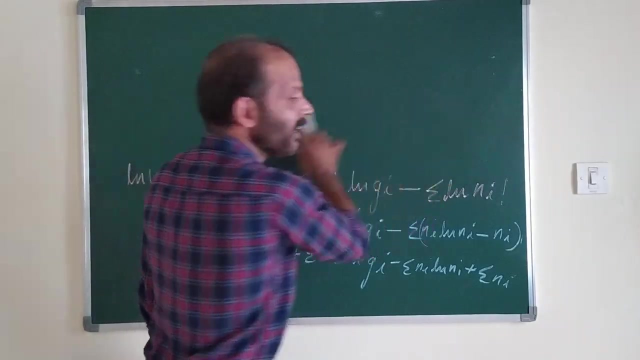 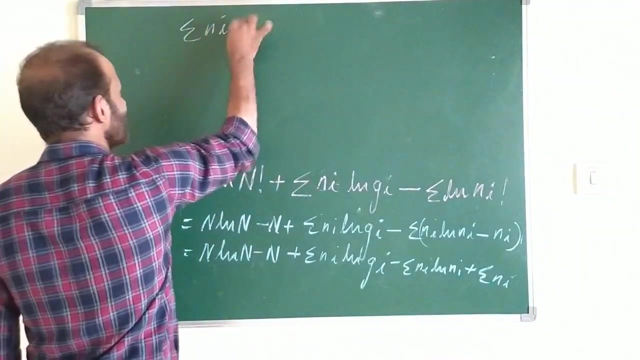 and I. so the equation we don't n? ln n minus n plus Sigma n I. LNG I minus Sigma n I. ln n I plus Sigma n I, but some of the n? I particles, that is Sigma n I. some of the n? I particles, there is Sigma n I, nothing but n. so we can replace this. 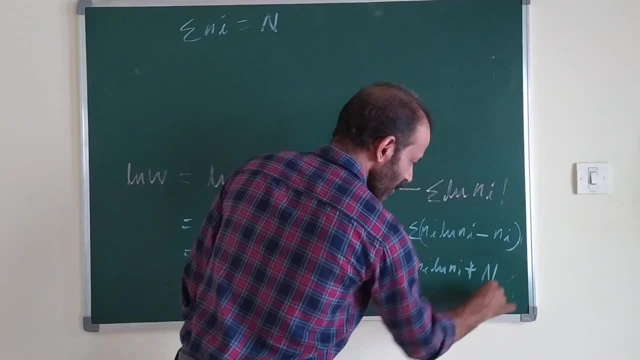 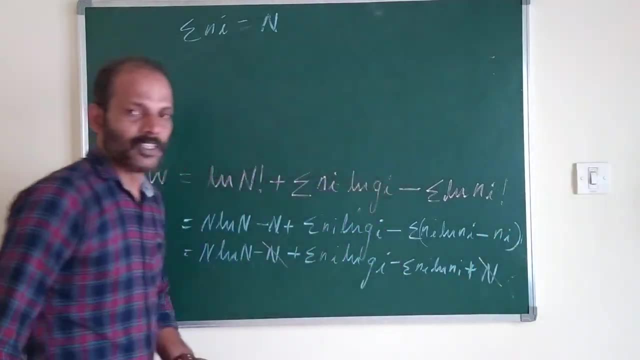 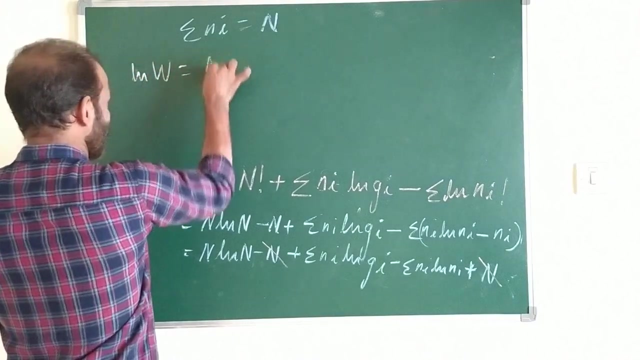 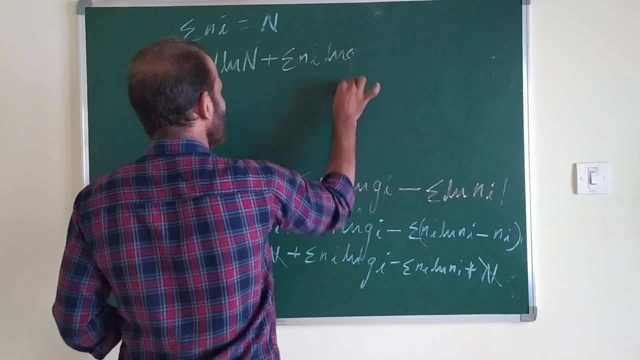 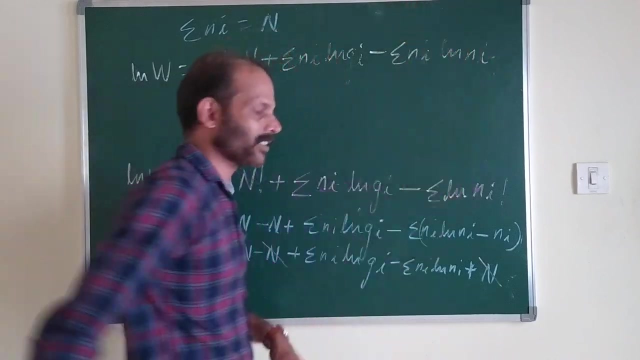 Sigma n I by n, so the equation become this one. so we can replace this Sigma n I by n, so the equation become this one. so this n minus n cancel each other, so we get the final next equation, as ln W is equal to n. ln. n plus Sigma n I, LNG. I minus Sigma n I, ln. that's our equation. 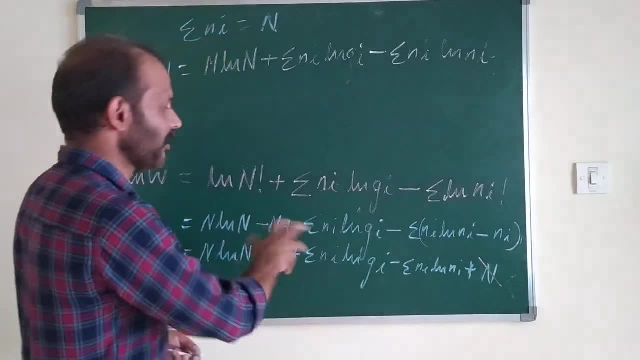 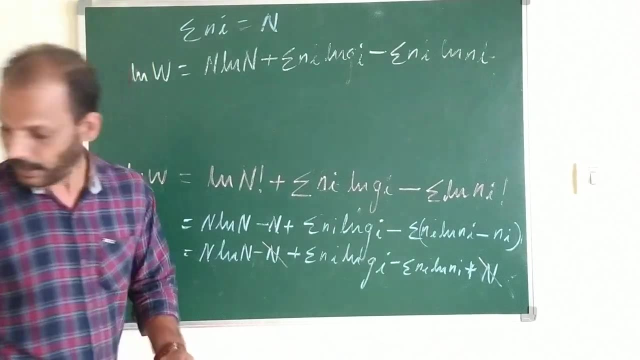 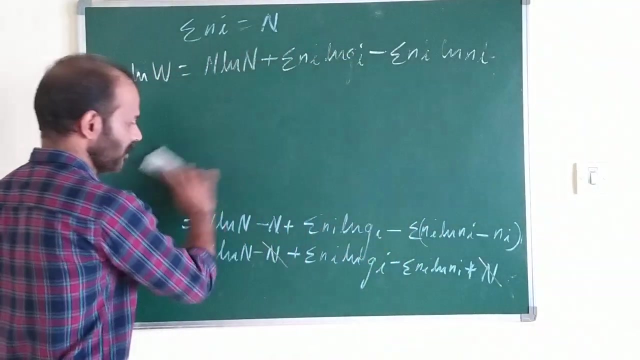 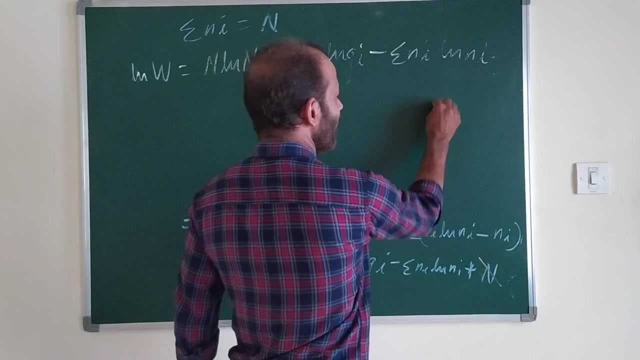 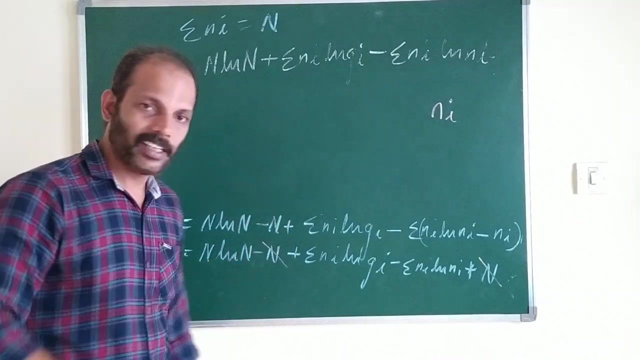 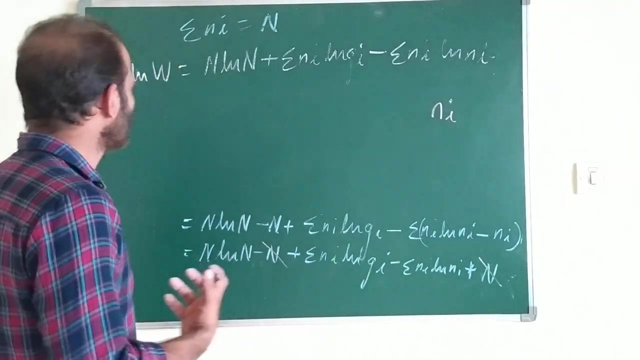 sir. next equation, after using sterling's approximation, then yeah, differentiating this, so number rates of the situation on that part. number of ways of distribution of n I less so desires the distribution of n I particles in aẻi an. energy levels with bgen was the gi. that's our aim. so we have to differentiate this one.